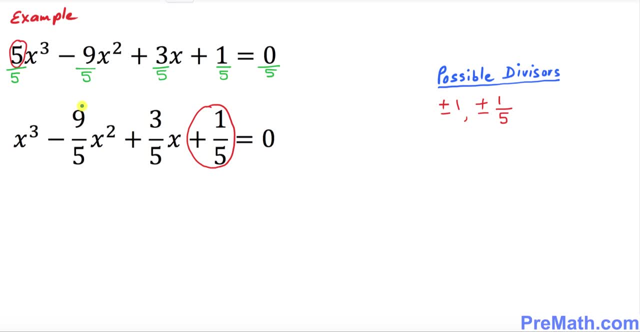 5.. One more thing: I want to just make sure that our highest degree of this cubic polynomial is 3.. 3 means that we must have at most three solutions. So that means we are looking for three numbers. So we're going to pick three numbers from these possible divisors If we add them up. 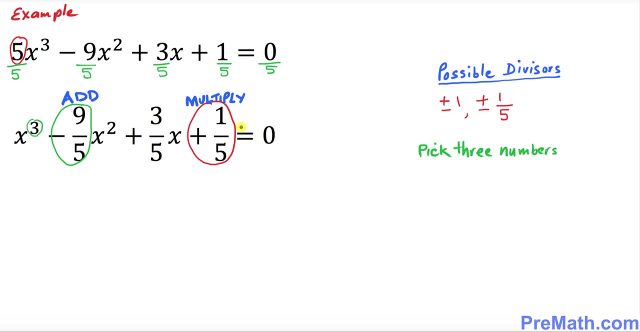 we must get this number. if they add up to this thing, If we multiply those three numbers, they should multiply out to 1 over 5.. So let me just show you really easy way to figure out those three numbers. Just focus on this: negative 9 over 5.. Negative 9. 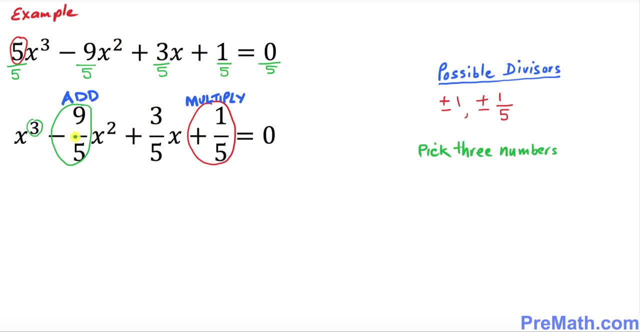 over 5,. 9 is pretty close to 10,, isn't it Negative? 10 over 5 is negative, 2.. So I can write this thing: negative: 9 over 5.. I can write as: isn't it this pretty close to 2?? So I can write negative: 2 plus 1 over 5, isn't it? So that is. 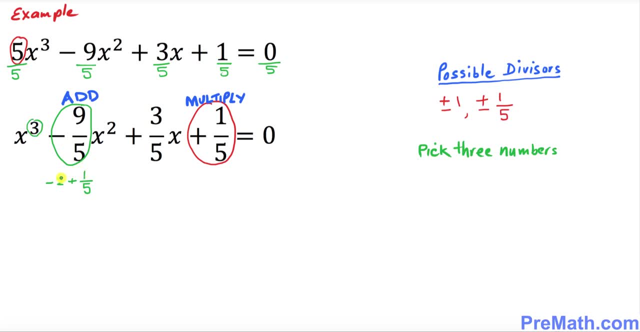 going to give you the same number over here, So that means over here. now what we're going to do is I'm going to put this negative 2. I can write as negative 1, negative 1 plus 1 over 5.. Since we are, 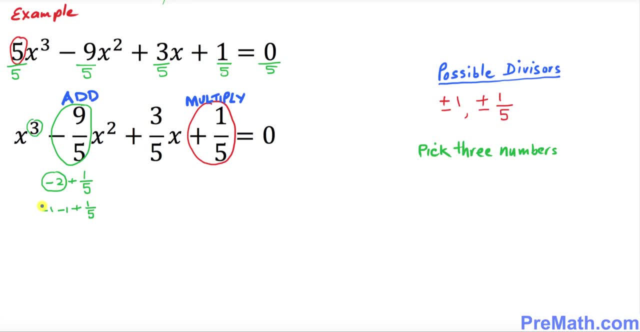 interested in three numbers right now over here. we're going to put this negative 2 over here. So this is the one number, this is the second one, this is the third number. If you add them up, we're going to get this required number And if you multiply them, obviously we're going to get. 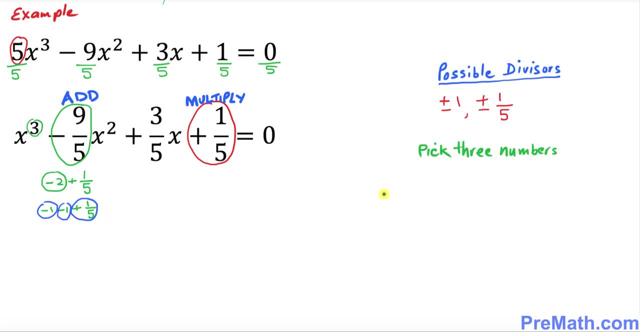 this thing. So that means we figured out over those three numbers. Those are negative 1, negative 1 and positive 1 over 5.. Once again, let me just repeat: if you multiply these three numbers, see that that is going to give you this one. and if you add them up, that should give you this. 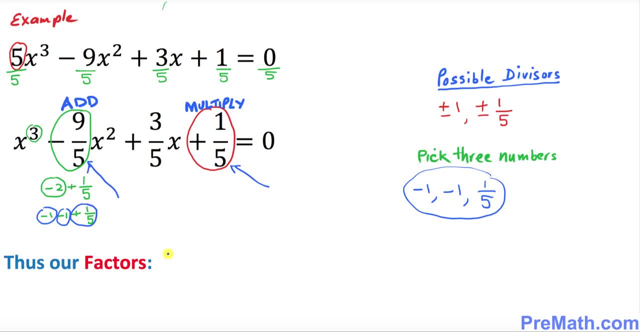 number. So thus our factor is going to be simply: let me just put down three parentheses. Let me just show you how we're going to do this thing. So you put down x, x and x. Now I want you to just put this number- negative 1- right up here, and this next one: negative 1 right up here and positive 1. 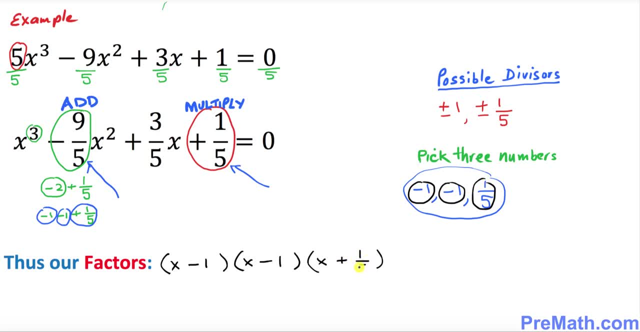 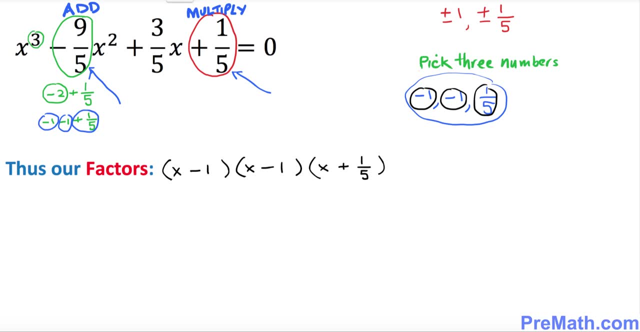 over 5 is going to be right up here. So the next thing, what we want to do is: I want you to just look at this part. This is a fraction. I want you to get this 5 and drag it to the front, So that. 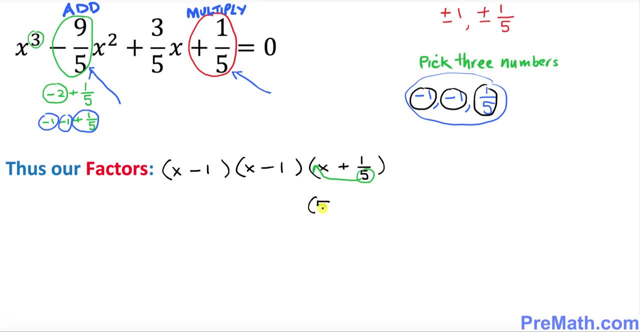 means this is gonna look like five X plus one. So our complete factors turns out to be X minus one times X minus one times this one, and that is our F. And finally, our solution set is gonna be a. simply, whatever, you got these numbers over here. 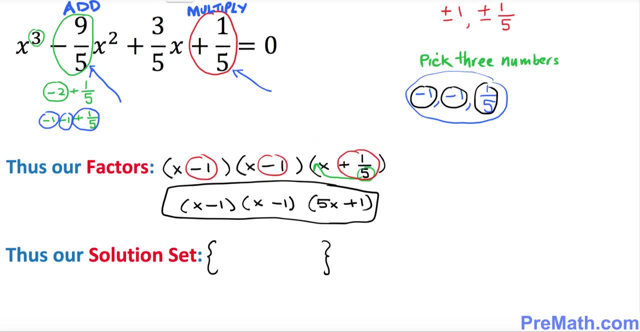 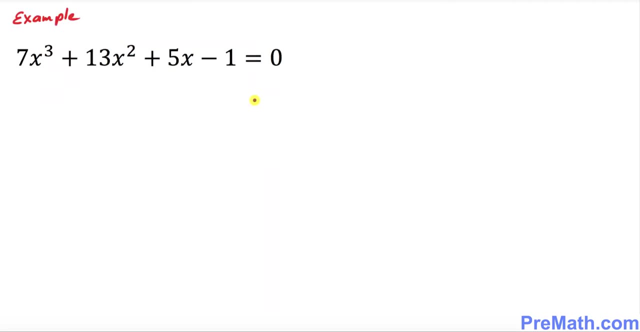 you see, right now you just switch the sign, change the sign, and that's gonna be our solution: set This become positive one, this become positive one and this become negative one over five, and that is our answer. Now let's focus on our second example. 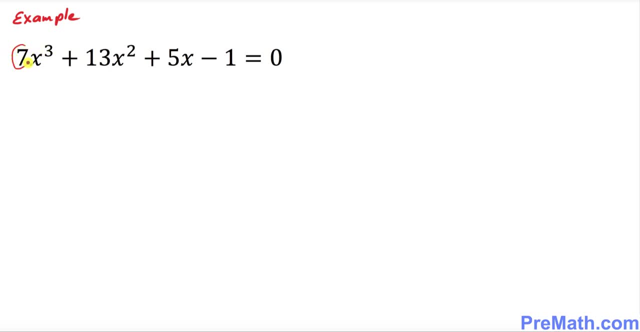 In this example. you see, our leading coefficient is seven. We wanna make sure that this must be one, So the best way to make it one is by dividing by two. So we divide by seven the same number. If we divide this one by seven, 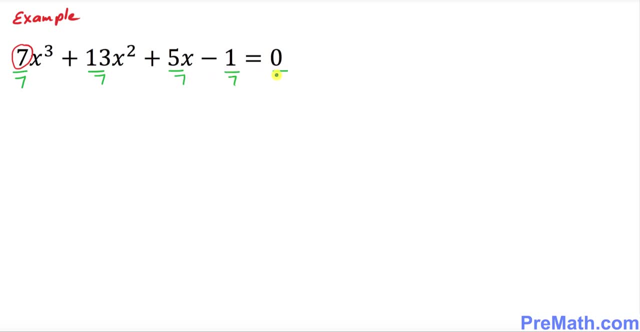 we must divide by seven across the board. So our problem is gonna look like now, with a coefficient one, leading coefficient one. Now I want you to just focus on the very last number, which is negative, one over seven. We wanna figure out the possible divisors of the factors. 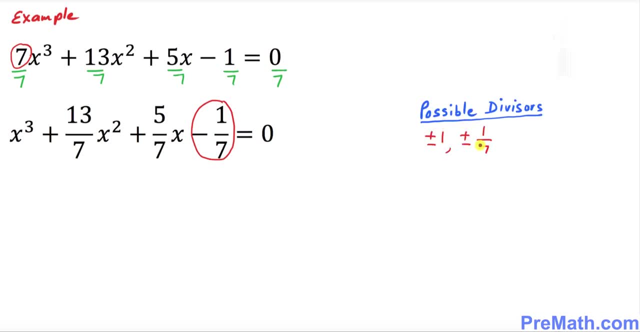 of this number. This our problem. The possible divisors turns out to be a positive and a negative one, and positive or negative one over seven. for this number, You can see this one, And now the next step is so we need to pick three numbers that, if we add them up, 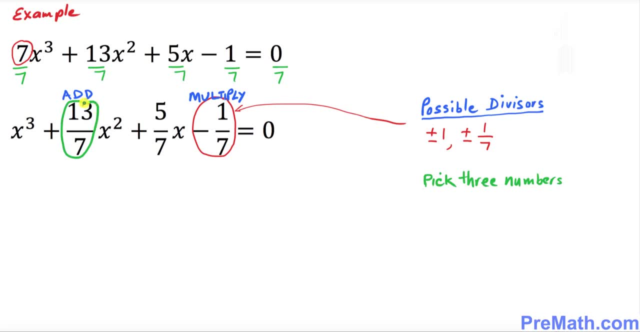 this adds up to this number. And if we multiply this, multiply this, multiply this, it multiplies up to negative one over seven. So there's many different ways. Let me show you an easy way to figure out those three numbers. So I want you to just look at this: 13 over seven. 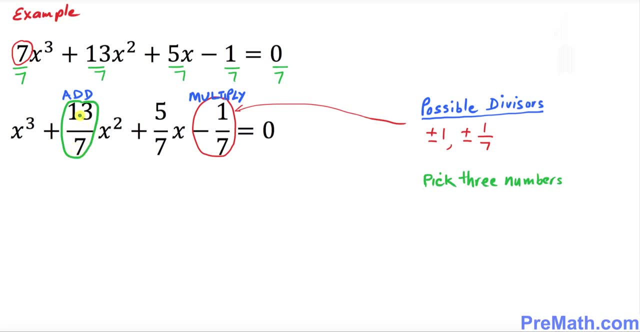 Let's manipulate it a little bit. Let's 13 over seven. This fraction could be written as two minus one over seven. That's gonna give you this one. Now I want you to just focus on two, And two could be written as one plus one minus one over seven. 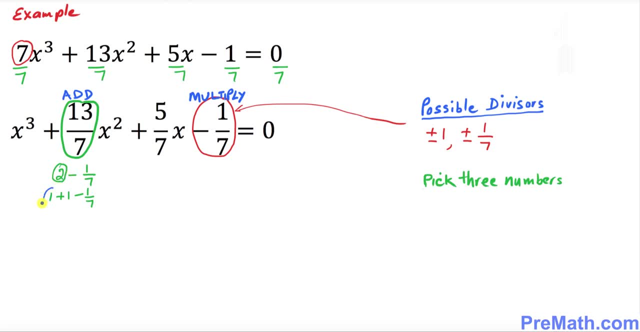 That means we got these three numbers. We needed three numbers. That's the first one, This is the second one, This is positive one, by the way, And this is the third one. So these are the three numbers, which are one, one negative, one over seven. 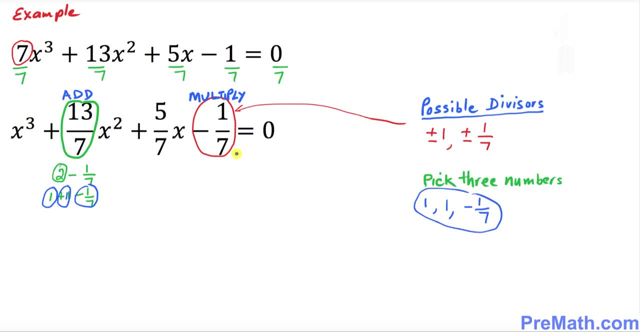 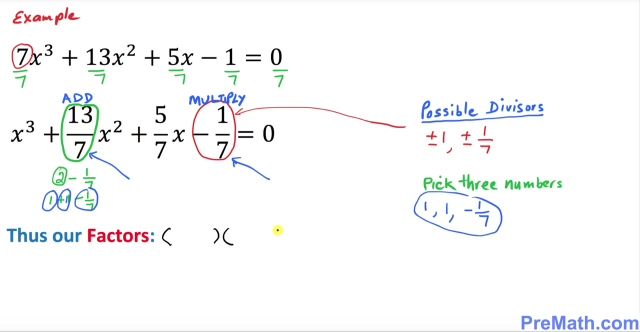 If you multiply them, we're gonna get for sure, we're gonna see that we get this number. And if we add them, we're gonna get this number. So thus our factors turns out to be. I want you to just put down three parentheses. 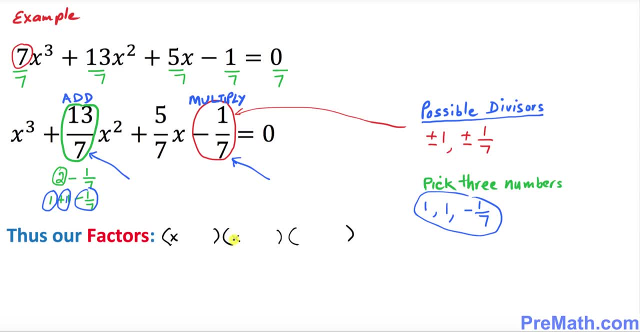 because we have three factors: x, x, x over here. Now I want you to look at this thing. This is a positive one. You put down positive one right up here, And there's another one positive one over here. I want you to put down positive one. 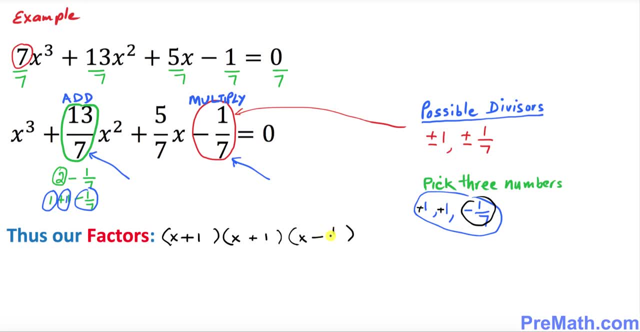 And this is the other one. It's negative one over seven you've put down. So those are our three factors. Now, this is a fraction. We wanna put it in a little bit different way. Okay, this seven at the bottom. I want you to drag it up to the front.